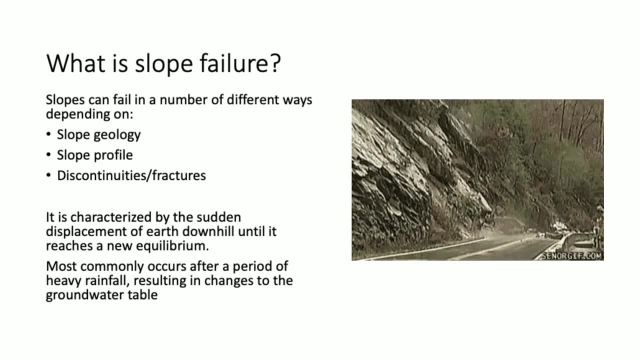 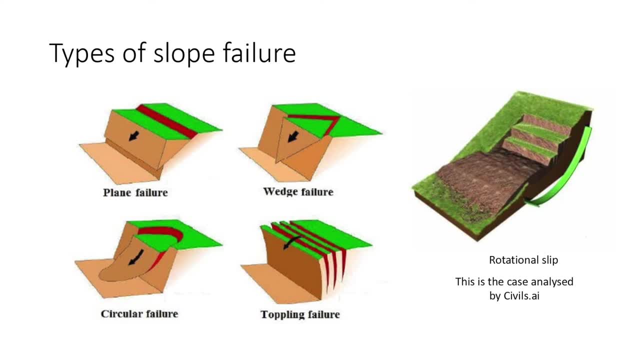 If a slope is susceptible, then failure usually occurs after a period of heavy rain which results in changes to the groundwater table. There are a wide range of slope failure mechanisms. Here we cover some of the most common failure types. Plane failure commonly occurs when discontinuities through the slope. 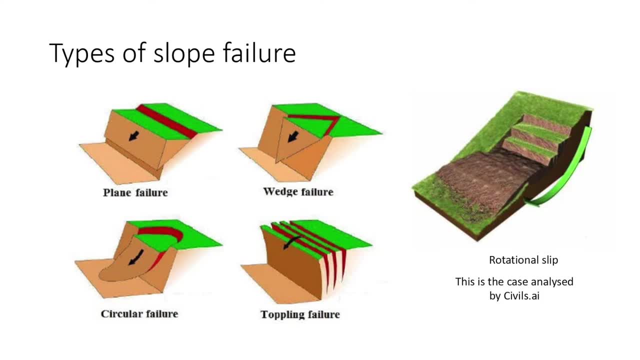 intersect to form a planar surface along which the block is free to move. Which failure occurs when two discontinuities, Discontinuities intersect whose lines of intersection are approximately perpendicular to the strike of the slope and dip towards the plane of the slope. 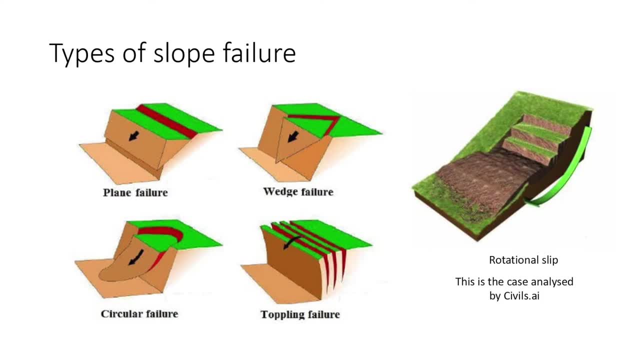 Circular failure follows a similar principle to wedge failure. Toppling failure occurs when columns of rock, formed by steep discontinuities, rotate about a fixed point at or near the base of the slope, followed by slip between the layers. Rotational slips are the most common form of slope failure and follow a circular arc through the soil. 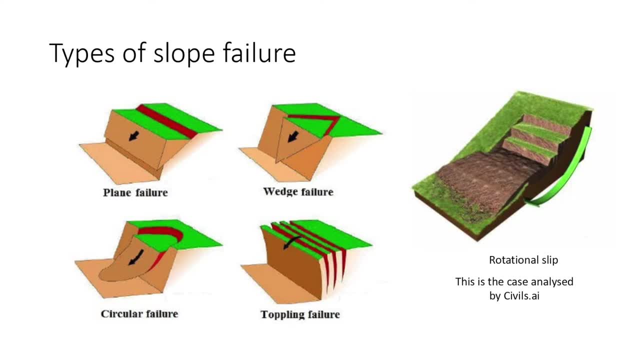 Translational slips are also common, Which are typically found when the top soil layer is underlain by a soil of very different strength. Further details on rotational slips will be covered in a later video. Sibylsai analyzes the rotational slope failure case. 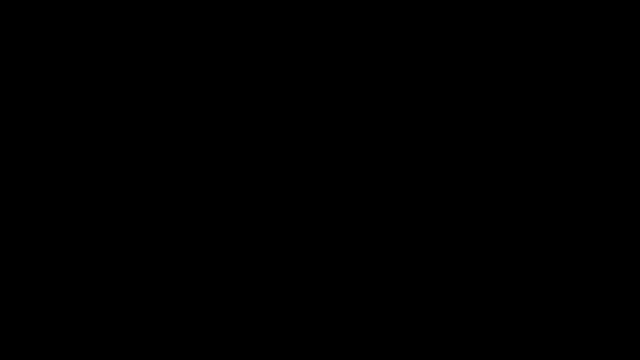 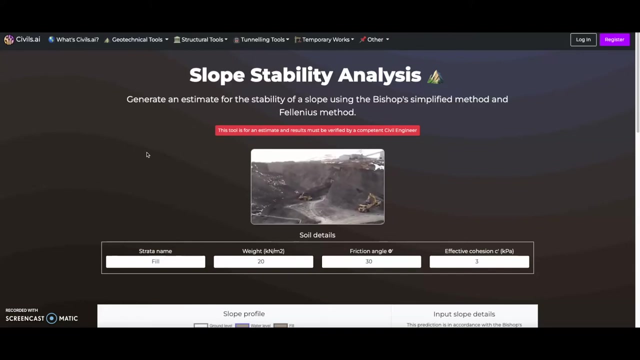 There are three types of rotational slope failure. Now let's look at how to use Sibylsai to calculate slope stability. In the first section we input our soil properties, We assume homogenous soil throughout the entire slope, and then we use the rotational slope to calculate the slope stability. 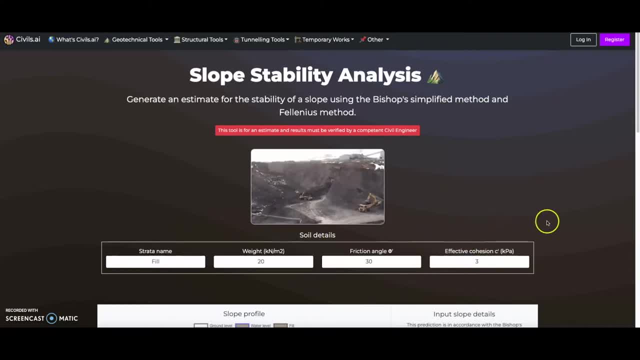 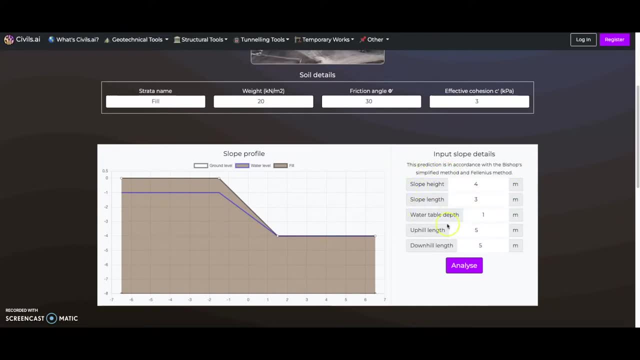 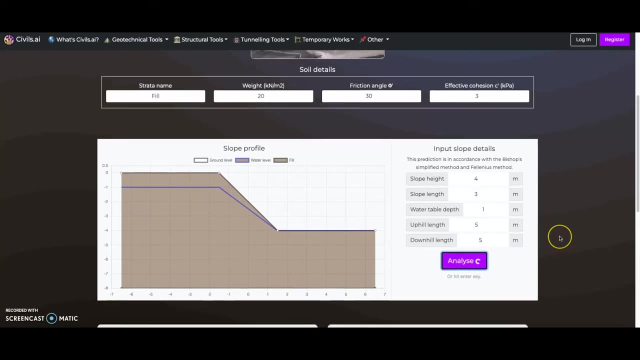 That long-term drain properties govern the analysis. Next, we can modify the slope profile. We can control the slope height, length, water table level and uphill and downhill lengths. After we are satisfied with our model inputs, we can hit analyze or the enter key to run the analysis. 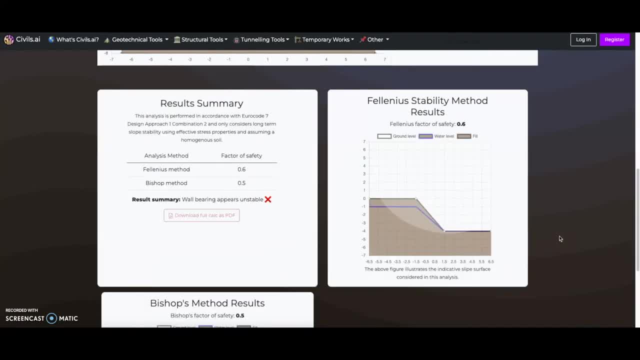 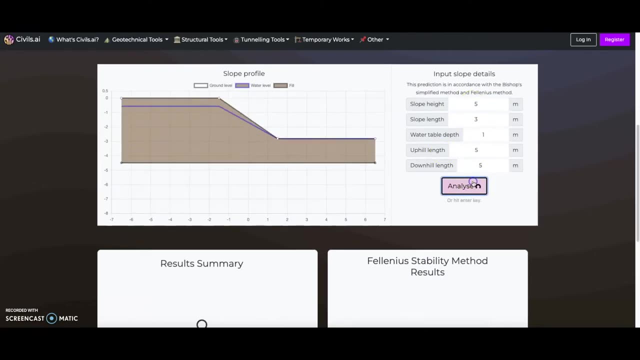 Our results will present the predicted factor of safety for this slope, using both the Felinius and the Bishop's simplified approach to calculate slope stability. The illustrations indicate the envisaged slope failure surface. We can further modify the model properties and hit analyze to recalculate and generate more results. 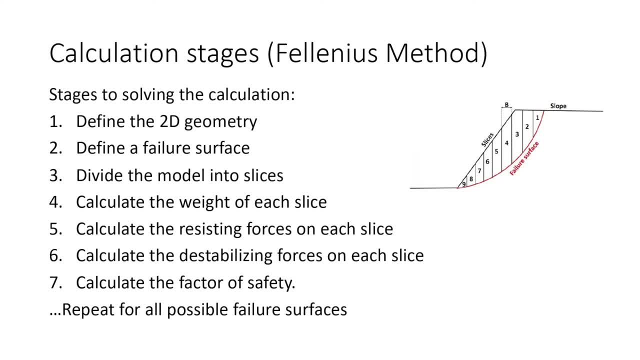 Let's now take a look at how we are calculating slope stability. We use seven calculation stages to determine a slope stability factor of safety. First, we need to define the 2D geometry, considering things like slope, height and length. Next, we define a failure surface which we assume the slope is failing along. 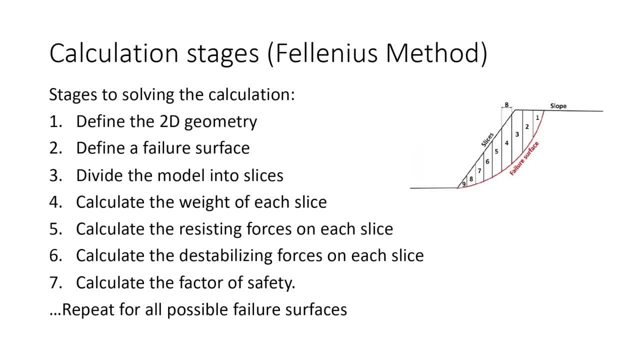 We split the model into a number of different slices. The greater the number of slices, the more accurate the calculation. We calculate the weight of each slice, Then calculate the resisting force on each slice, Then calculate the destabilizing force on each slice. 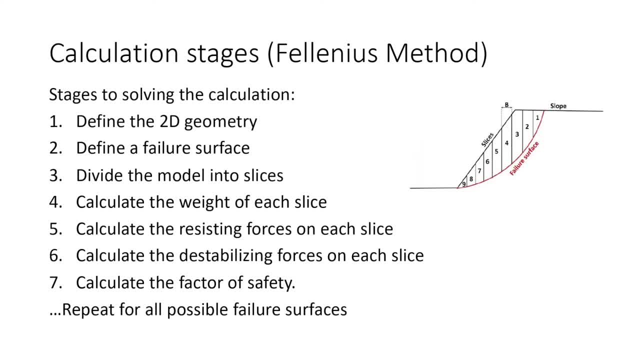 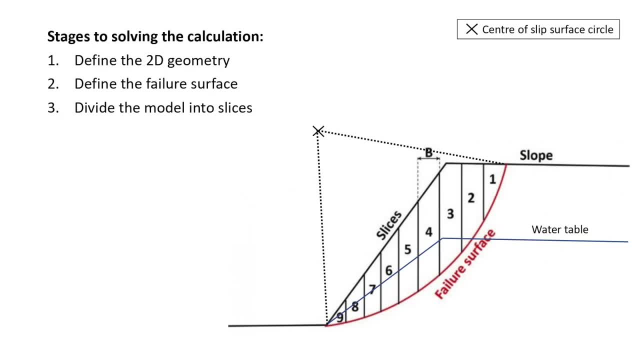 Finally, we calculate the factor of safety between resistance and destabilizing forces. We repeat this process for all possible failure surfaces. Let's look at stages 1 to 3.. After defining the 2D geometry and water table level, we assume a circular failure surface through the slope. 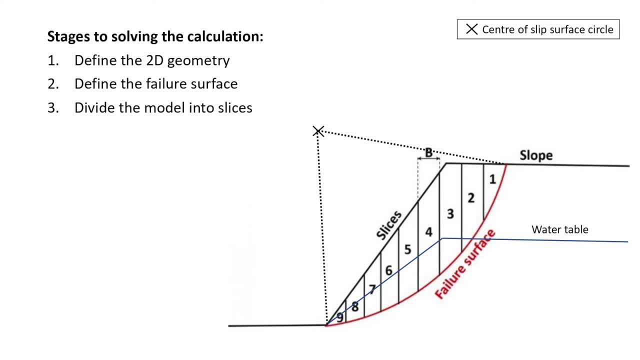 For now, we can define the center of this failure slope and radius at an arbitrary location. We then divide the slope, within the bounds of the failure surface, into a number of slices, the more the better. After we have split the slope into a number of slices, we can consider these slices individually. 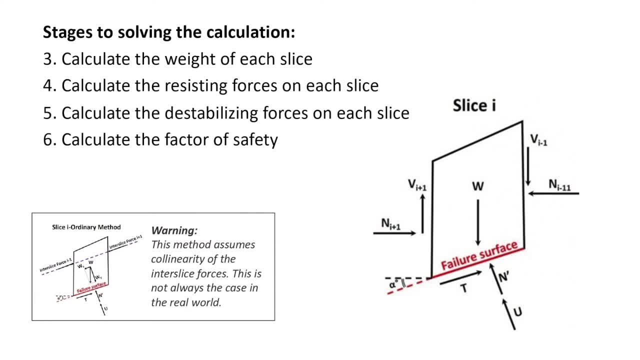 Each slice follows the slope at an angle alpha. Each slice has a weight, normal force and water pressure. There is also shear resistance acting on the slope, base, T, and vertical shear resistance between each slice, V. This calculation uses the Felenius approach, which assumes the interslice force and resolves to zero for each slice. 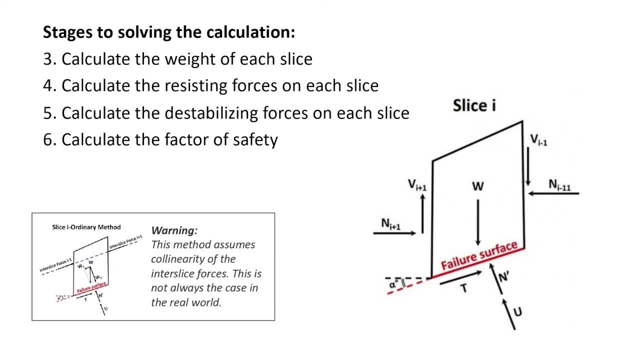 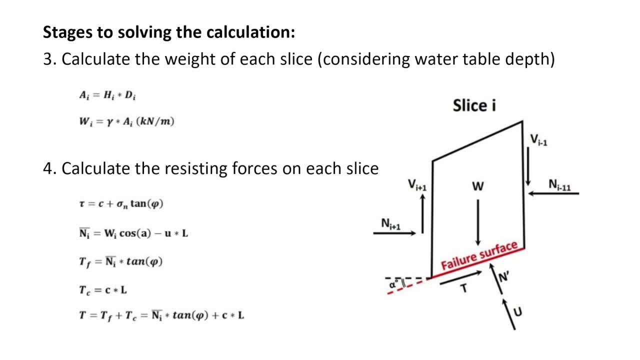 Please note this is a simplification and can lead to errors in some cases. The weight of each slice is calculated using the density and area of the slice. Next we calculate the resisting forces on each slice. The calculation uses the Mohr-Coulomb failure criterion to calculate the shear resistance. 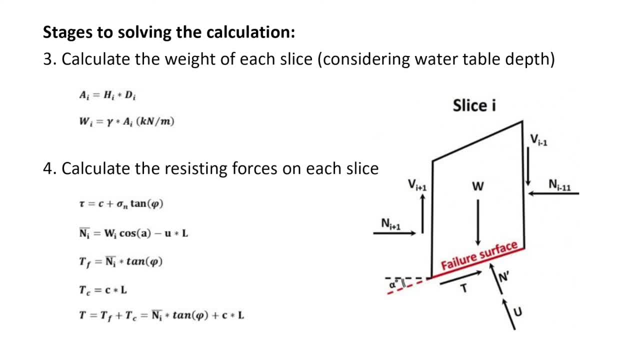 This equation uses the cohesion normal force N and friction angle. The normal effective force N I is then calculated for each slice considering the weight angle, pore water pressure and arc length of the slice base. The corresponding friction force is calculated using the effective normal stress and the friction angle. 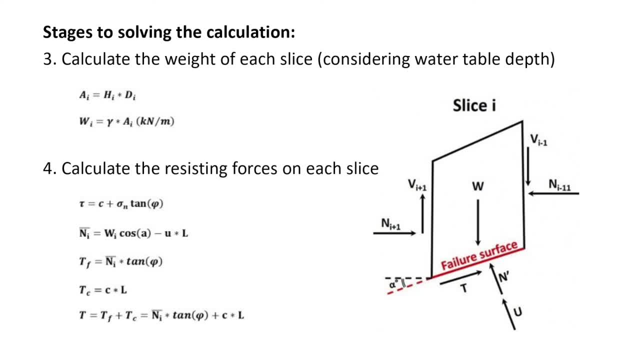 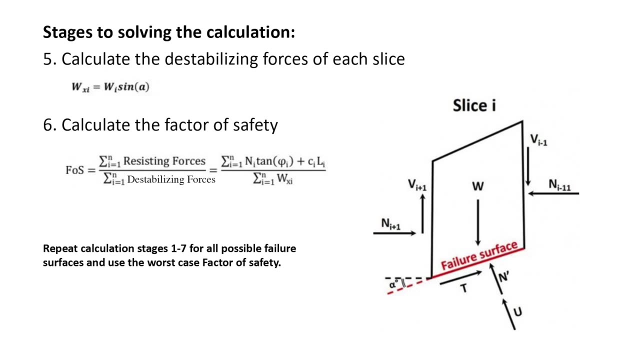 The cohesive resistance force is calculated using the cohesion and slice length. The overall resistance is calculated as the sum of the friction and cohesion resistance. The destabilizing forces on each slice are calculated using the weight of each slice and the angle of the slice base from horizontal. 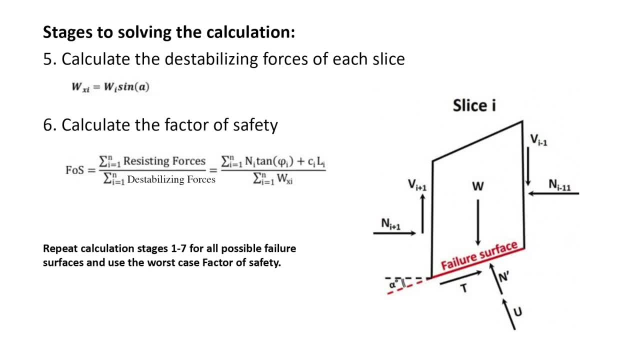 The factor of safety of the slope is the ratio between the sum of the resisting and sum of the destabilizing forces acting on all slices. Calculation stages 1 to 7 should then be repeated for all possible failure surfaces of the slope, with the worst case factor of safety then adopted.